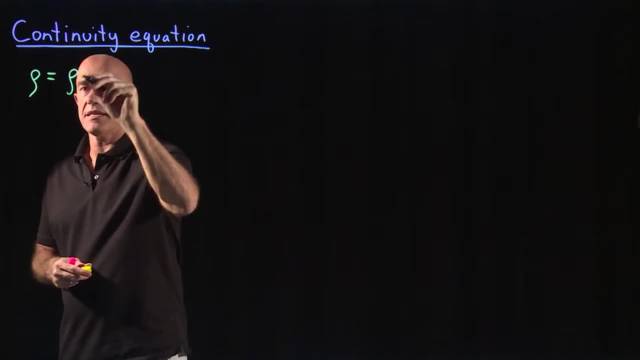 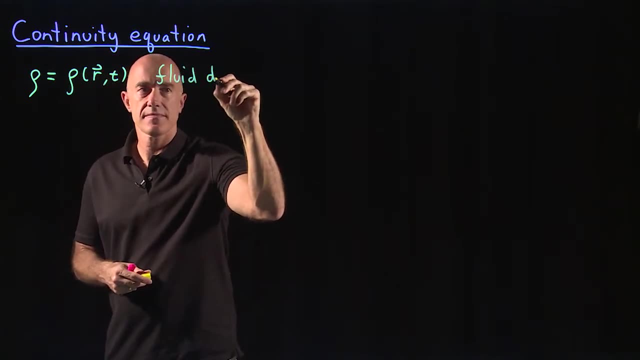 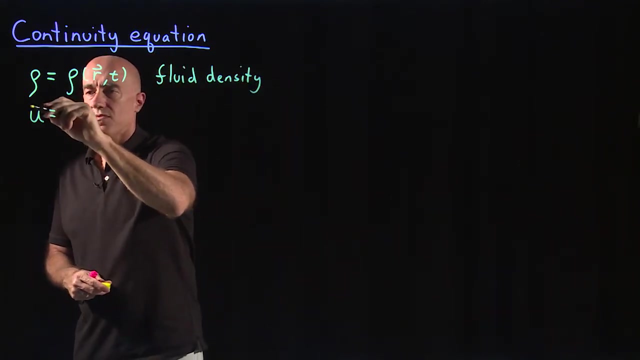 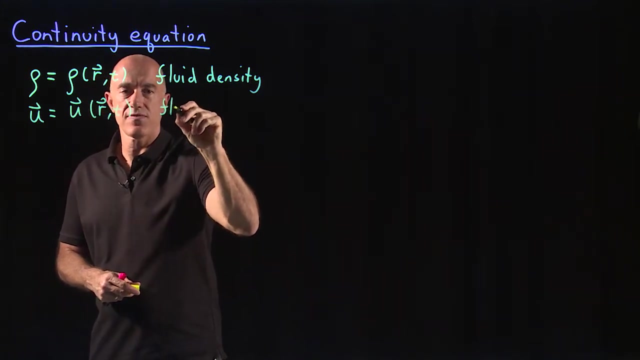 quantities. One is rho, which is a function of position in the fluid and time, That corresponds to the fluid density, The mass per unit volume. The other is u, which is a vector field, which is a function of position and time, And that corresponds to the fluid velocity right. 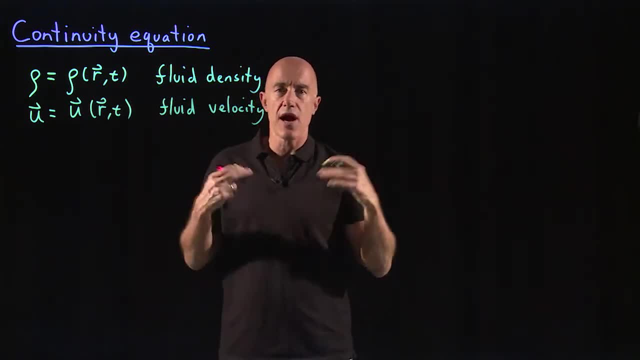 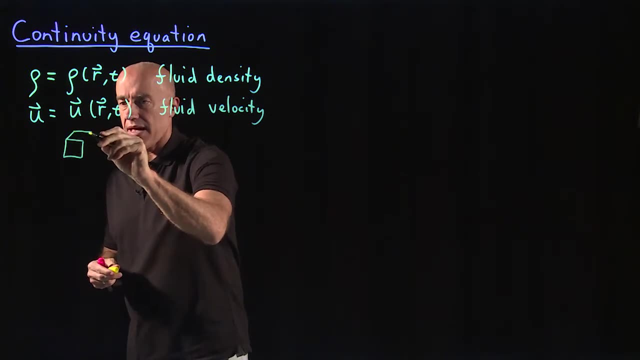 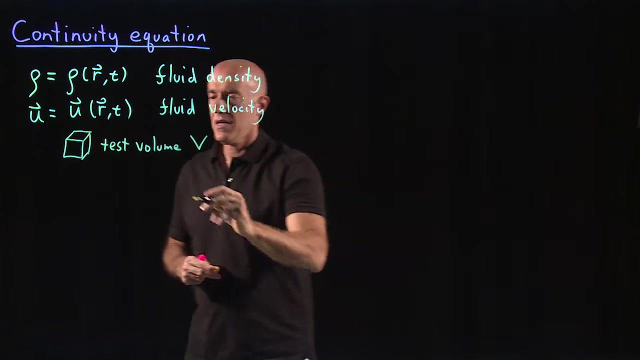 The length per unit volume, The length per unit time. Okay, to derive a continuity equation. you consider a test volume. It can be any shape, any size. So this is called a test volume And it's enclosed by a surface. So it's a test volume v enclosed by surface s. 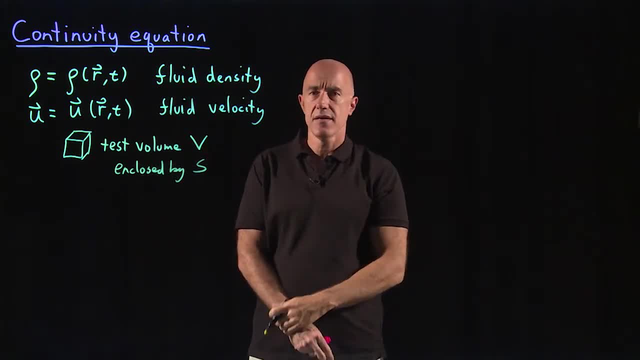 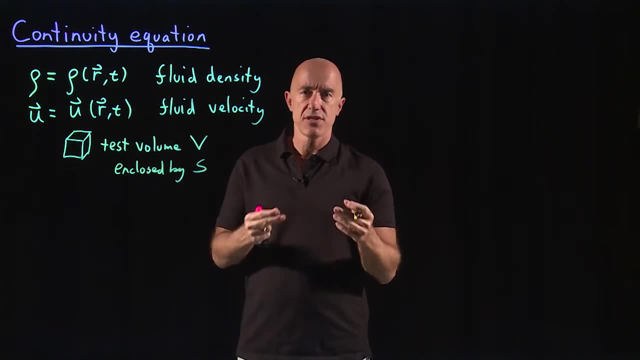 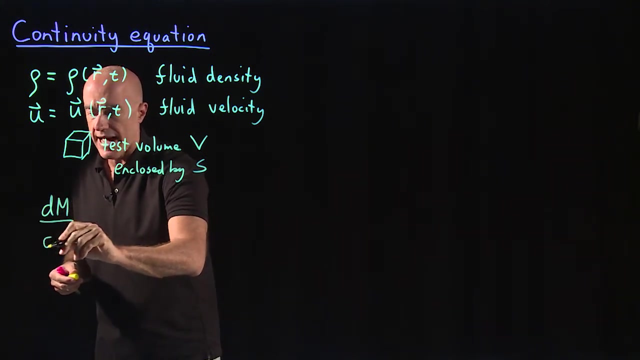 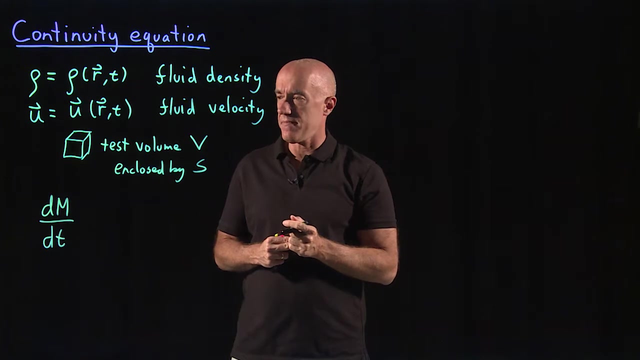 Okay, And then let's try and write then how the mass of the fluid in this test volume changes in time. So we're writing an equation for the dm dt, the derivative of the mass inside this test volume. as a derivative with respect to time, The mass of fluid in this 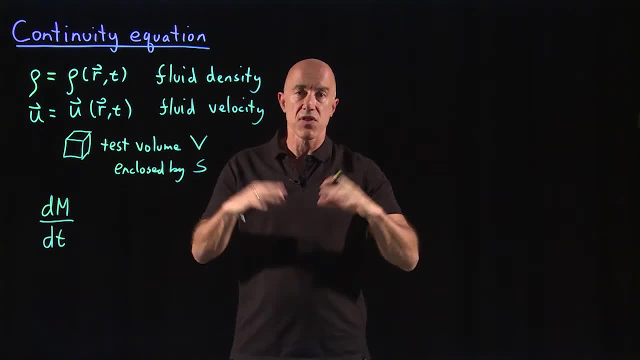 test volume changes because of the mass of the fluid. So the mass of fluid in this test volume changes because of the mass of fluid in this test volume. So we're writing an equation for the first took. This is a basic equation, So the line ofatenosing simulation is going. 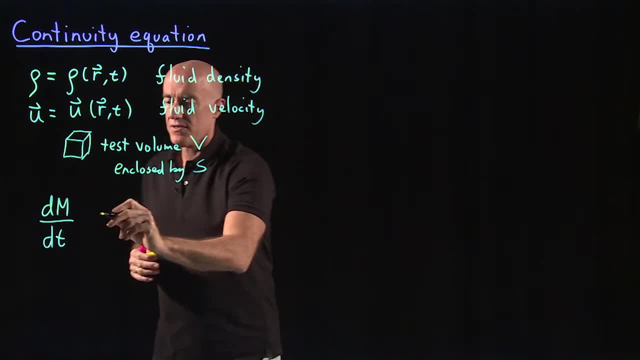 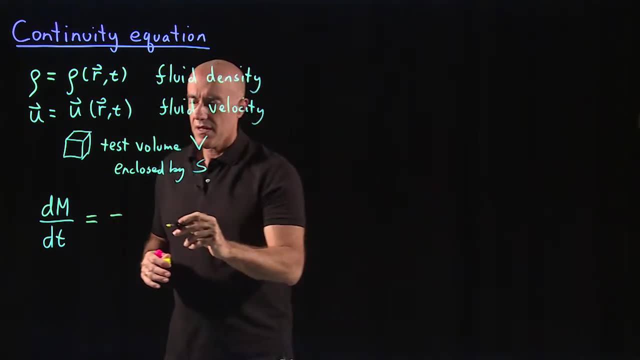 to give us h of time to here, And then you're going to get e through r, which, if we want to find h of time, then it would be n bar per square root of z, silver square root y. Then the answer is ea through r times u dot dA plus equal to and whenever the umbilical 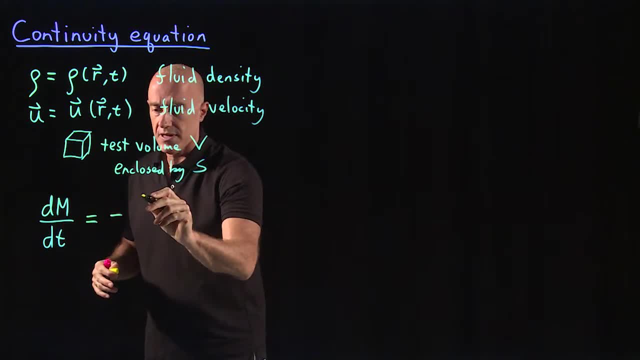 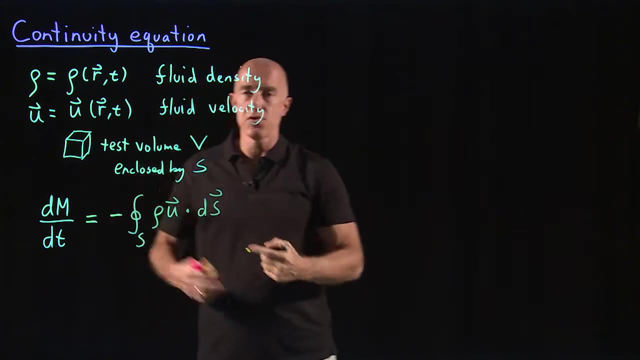 force of this test volume. So what happens to the? this must be dice. then we have the distance And all that stress is inside this test volume. The defense is dh of time 52. technical example of. So the units of this right-hand side is mass per unit time. 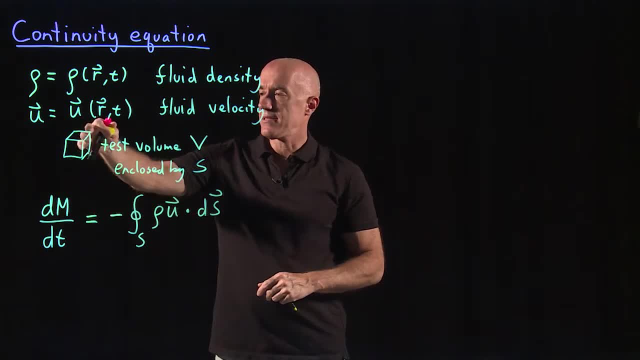 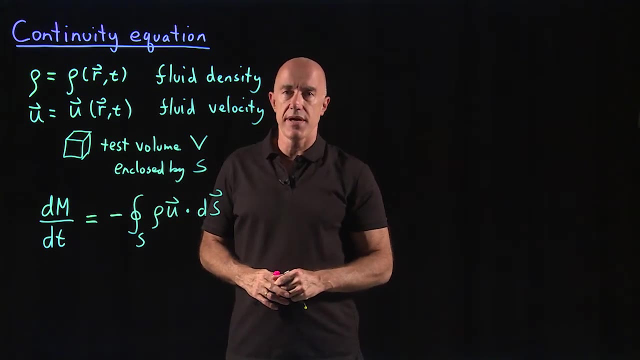 The left-hand side is mass per unit time And the time derivative of the mass in this test volume is equal to negative of the mass flux through the surface. okay, So this is essentially the continuity equation. We want to put it in a more standard form. 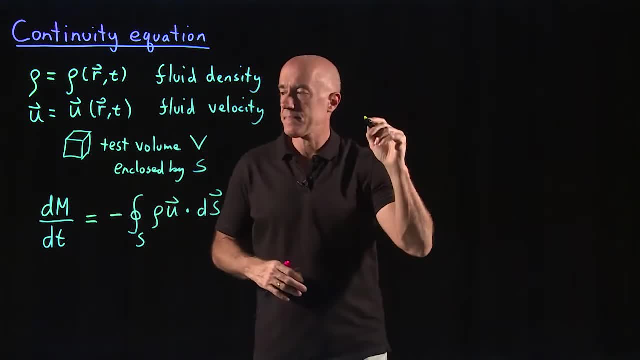 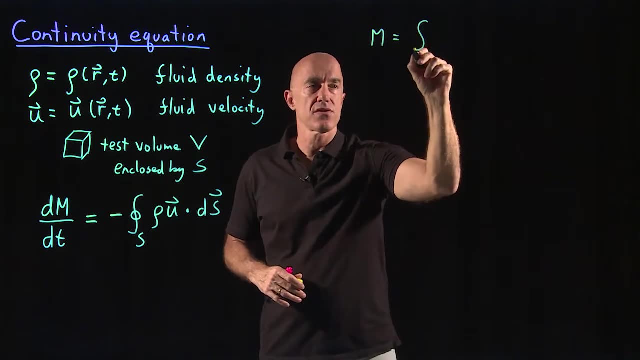 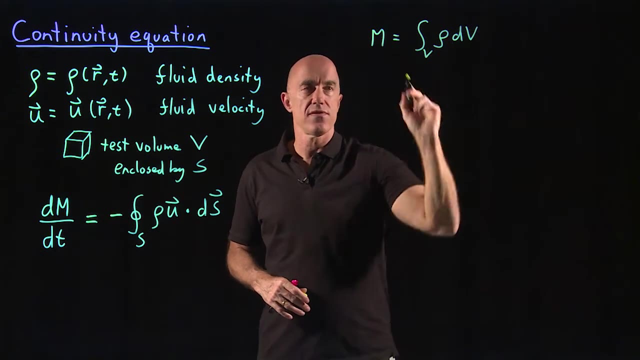 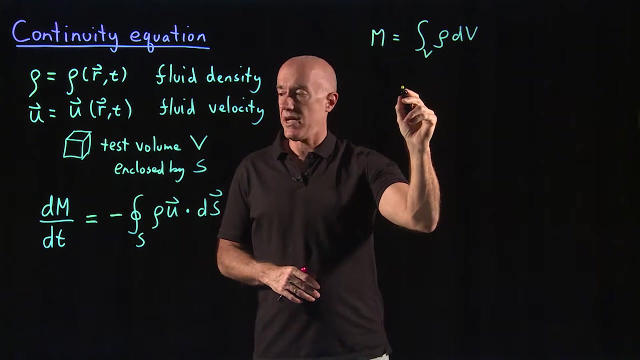 A more standard form would use m. So the mass in this volume is a volume integral over the density. dv, right, The mass per unit volume integrated over the volume. That's the left-hand side. So then if we want to write dm, dt. 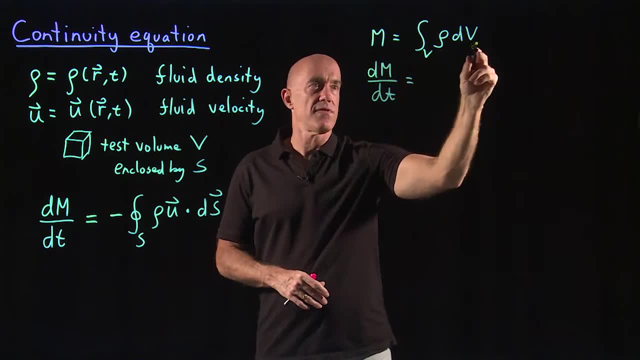 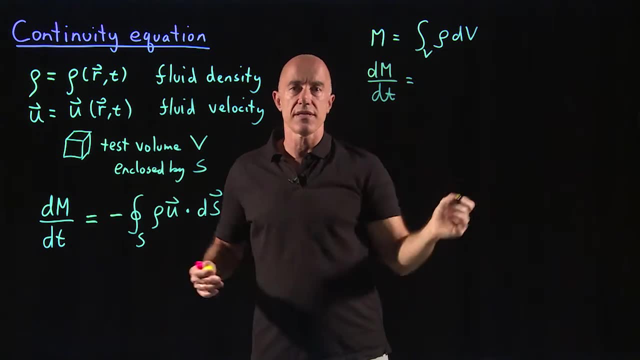 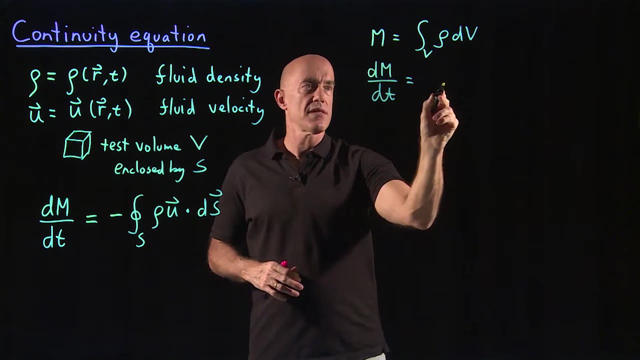 that's the time derivative of this. Rho is a function of position and time, but the volume integral that you're integrating over is independent of time. So we can bring the time inside of the integral. So that would be the integral over the volume. 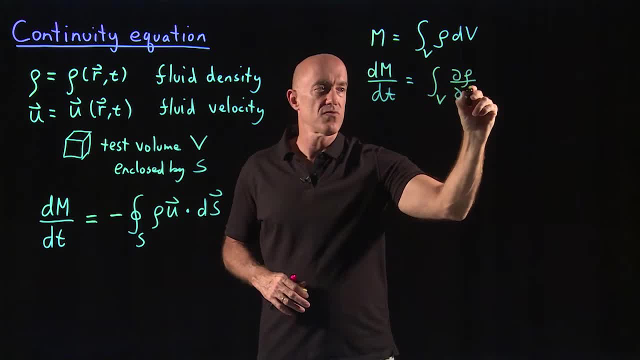 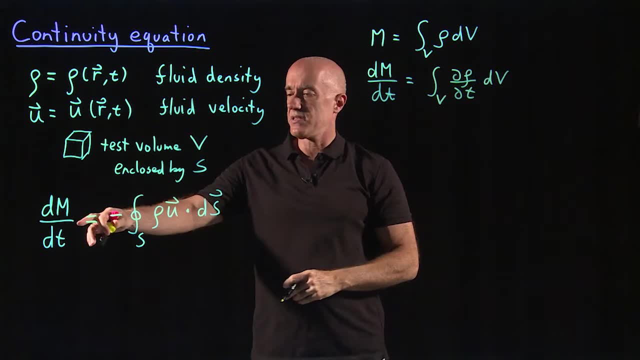 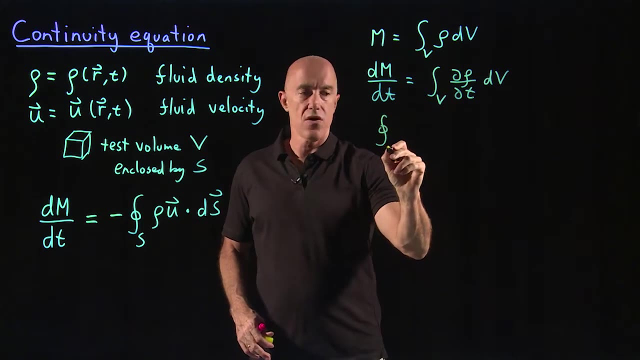 And we'll need to use a partial derivative here, because rho is a function both of position and time. Dm, dv. okay, So that would be the left-hand side. The right-hand side we'll use the divergence theorem, So we have the integral over the surface of rho. u dot ds. 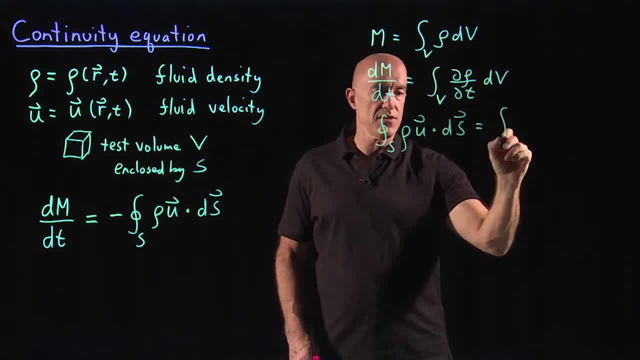 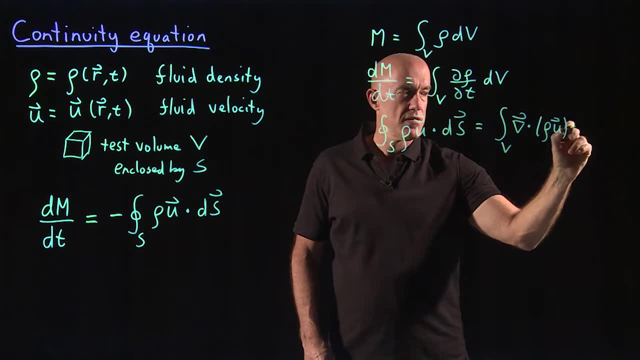 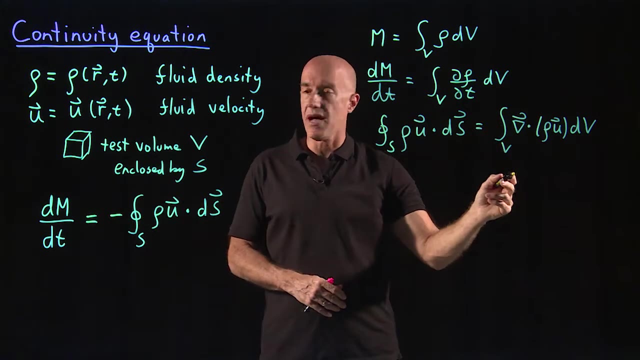 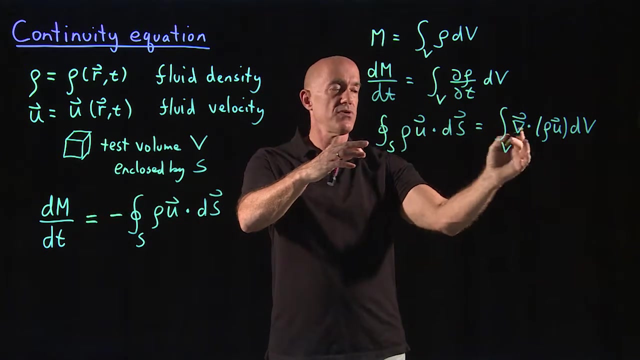 Applying the divergence theorem becomes an integral over the volume of the divergence of rho times, u, dv, okay, Okay, And that gets a minus sign on the right-hand side. So if we bring the right-hand side into the left-hand side and we use these two results so the minus sign on the right becomes plus on the left. 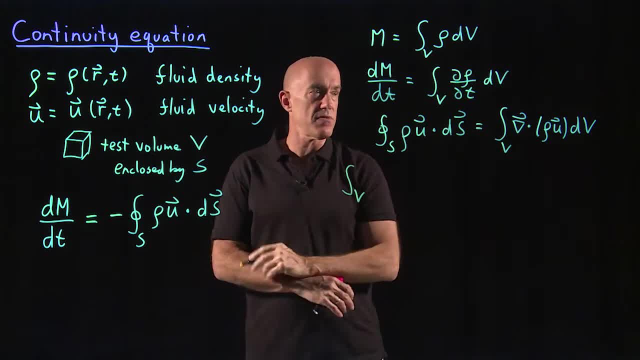 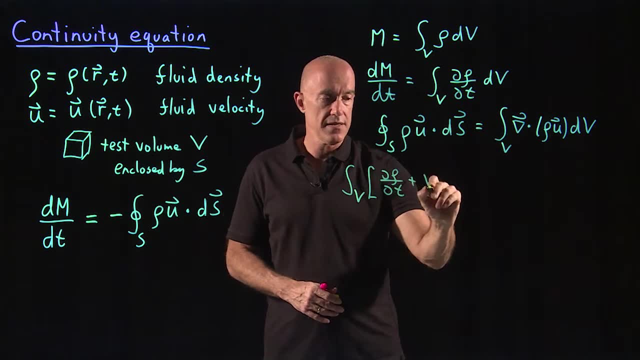 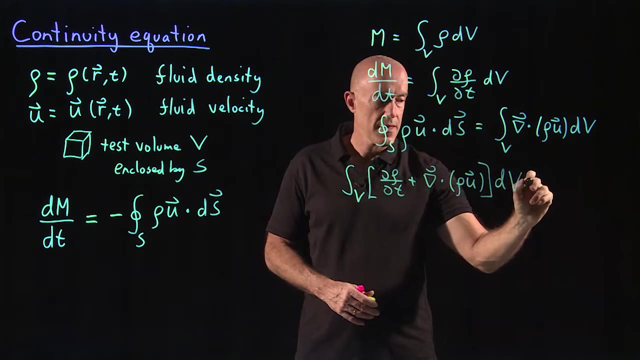 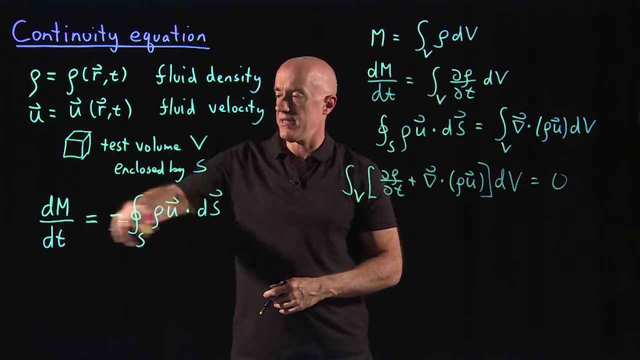 And put them all under one volume integral, we get the volume integral of d rho dt plus del dot rho u, And then we have the integral over the volume integral. dv equals 0, okay, So our continuity equation: dm dt equals minus the mass flux. 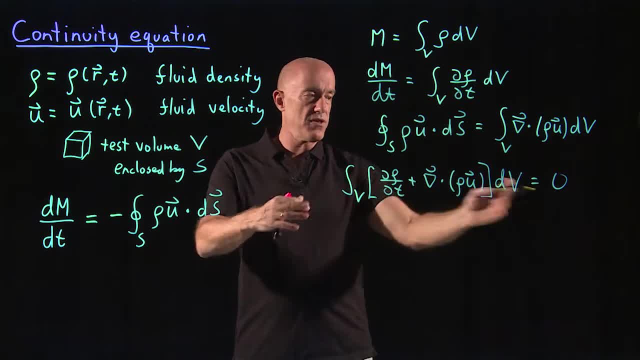 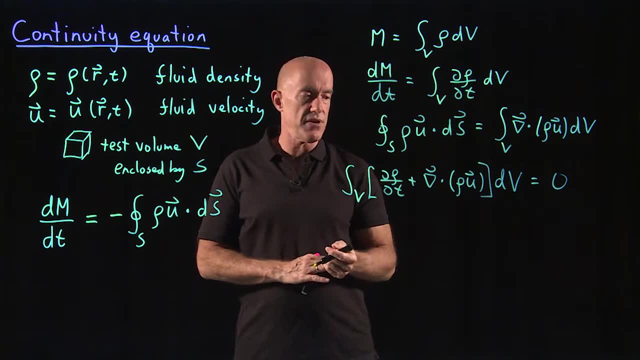 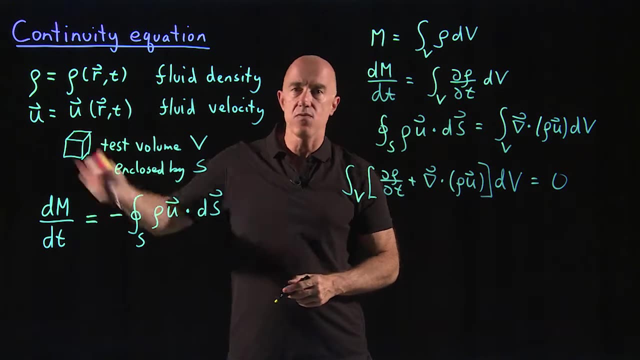 becomes a single volume integral. the volume integral of d, rho, dt plus del dot, rho, u, dv equals 0, by way of the divergence theorem. Okay, This is true For any test volume. the test volume can be anywhere in the fluid flow. 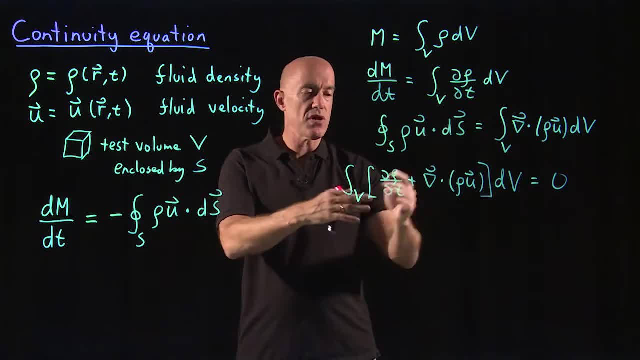 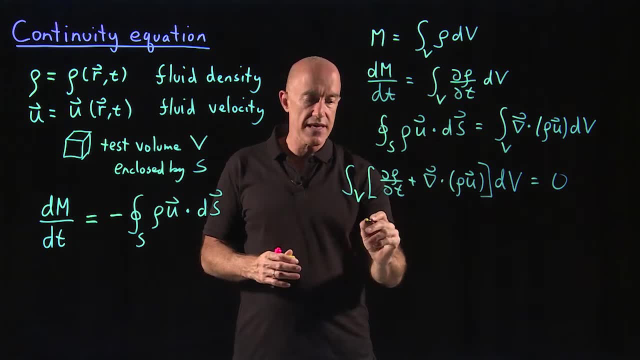 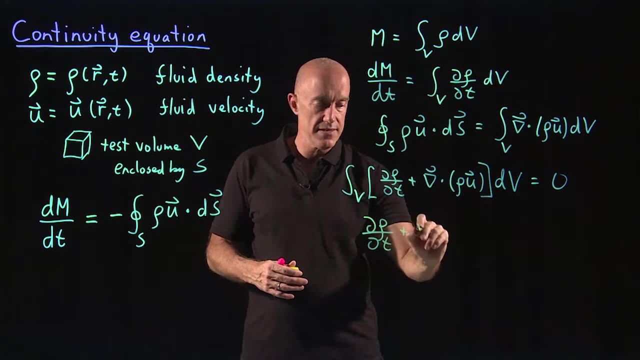 It can be any shape, any size. The only way this is true for all volumes v is if the integrand equals 0.. So that gives us the usual form of the divergence theorem, which is d, rho, dt plus del dot. rho u equals 0. 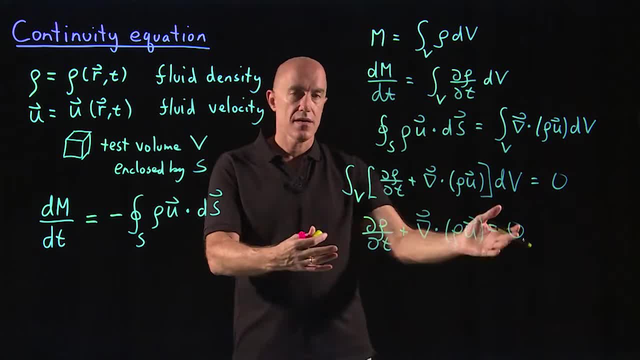 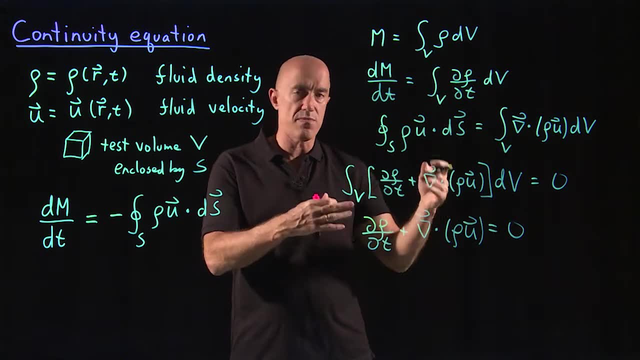 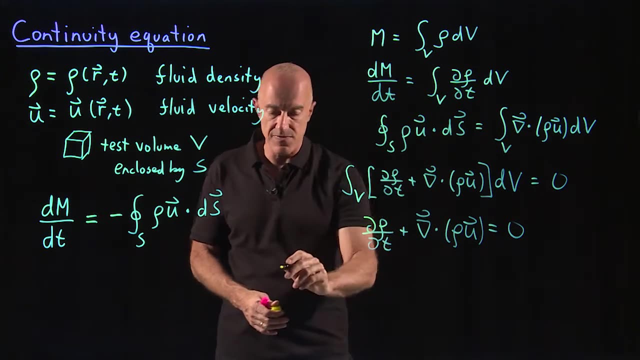 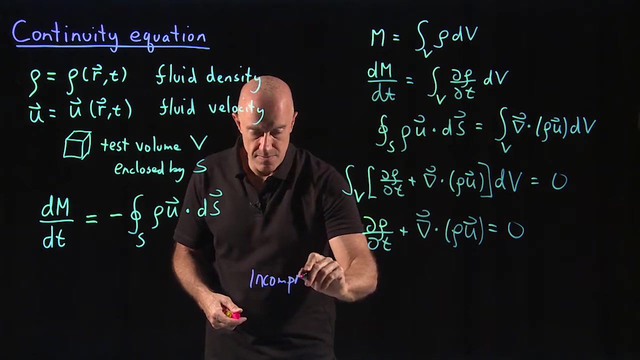 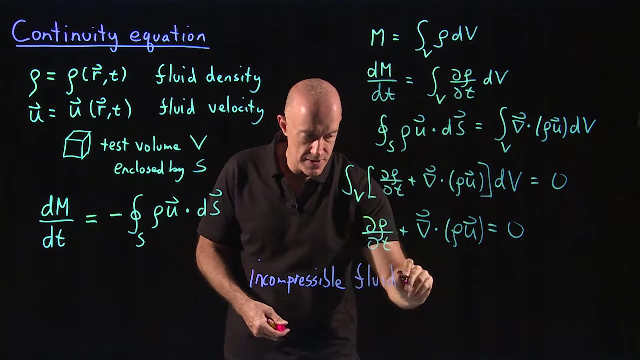 Okay, standard form for a divergence theorem, for a continuity equation: the standard form of the continuity equation. There's a special case that's called an incompressible fluid. So for an incompressible fluid, incompressible fluid we have, the density is a constant. okay. 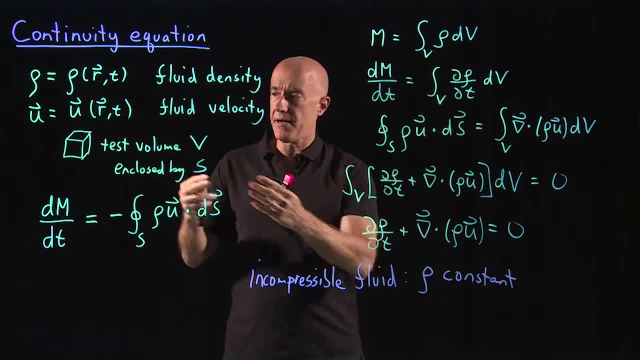 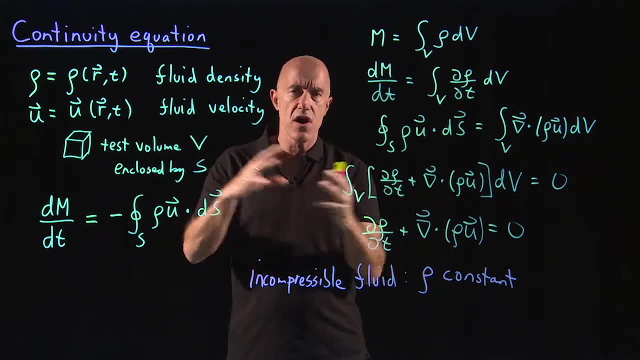 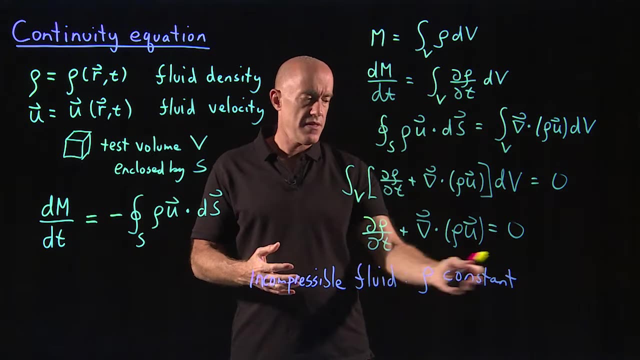 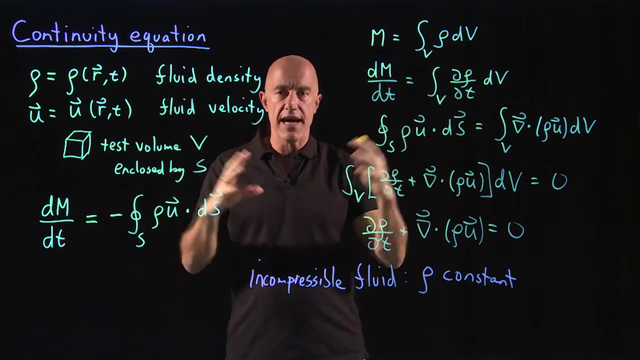 So a typical fluid such as a liquid is very hard to compress it. If you can't compress it, you can't change the density. So typically for a liquid the density is a constant. A gas is easier to compress. You have these tanks of compressed air. 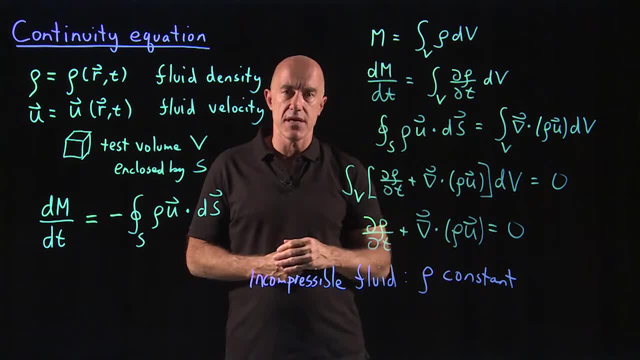 You can compress a gas. So for a gas sometimes this condition doesn't hold. But if rho equals constant d, rho dt is 0, then And rho can be pulled out of the divergence. So then we get the incompressibility. condition will be: del dot u equals 0. 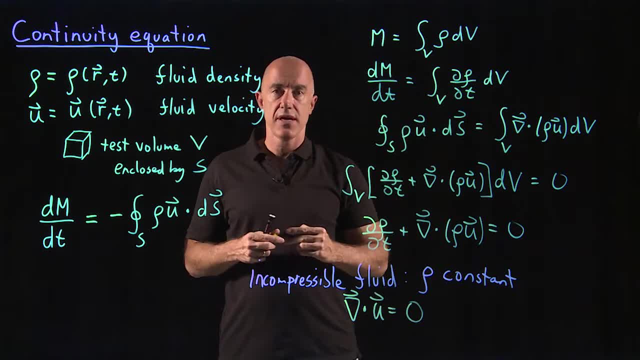 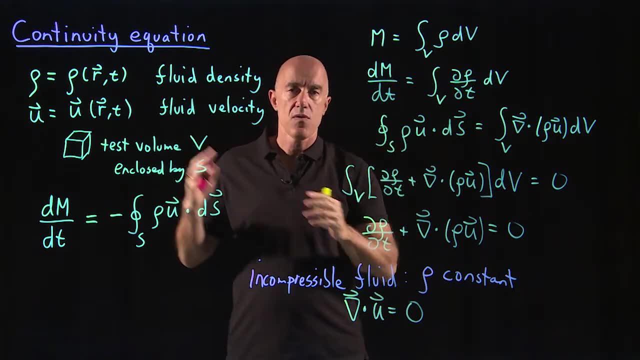 Okay, Okay, So del dot u equals 0,. okay, Del dot u equals 0.. Physically, what that means is that if you have some volume, whatever flows into the volume has to flow out. Okay, we'll see. that's the meaning of del dot u equals 0. 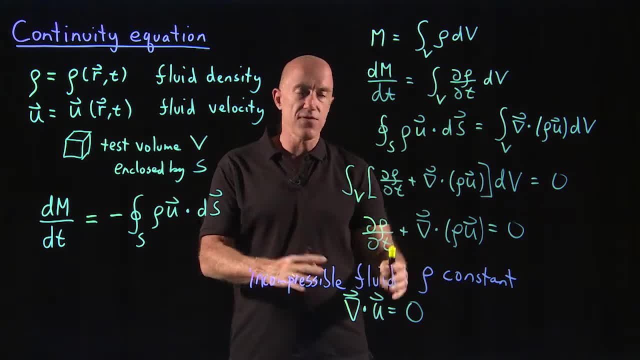 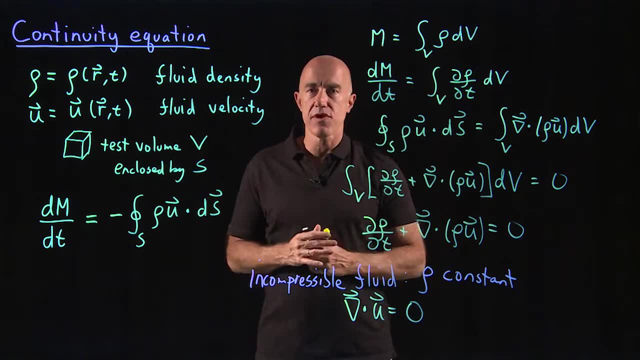 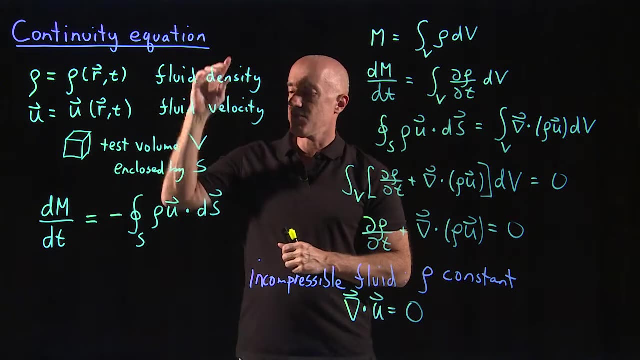 There are no sources or sinks of fluid, and fluid cannot get compressed inside of that volume. Okay, So let me recap. In this lecture, I derived the continuity equation for a fluid. The reason I'm doing it here is because the derivation converts this mass-flux.